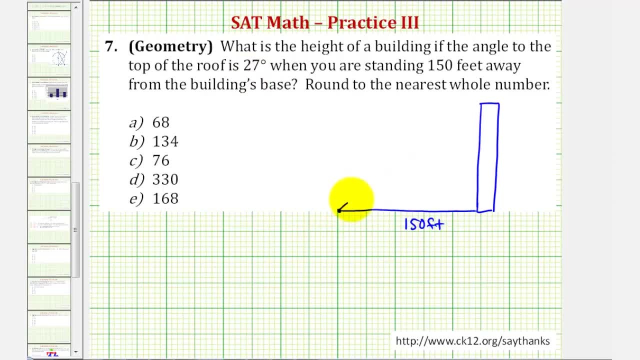 would be formed from this point to the top of the building, where this angle here measures twenty-seven degrees. Notice, we've just formed a right triangle, and therefore we can find the height of the building with the length of this segment here using right triangle trigonometry. 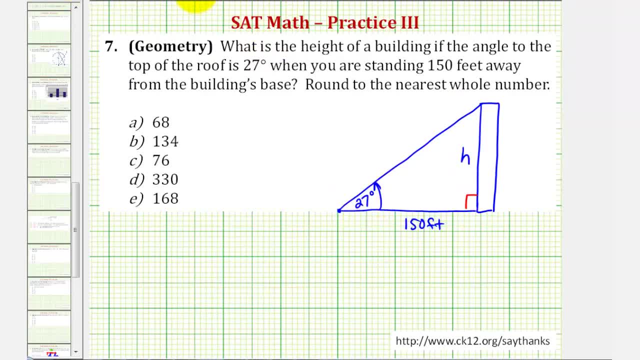 So for referencing this angle here that measures twenty-seven degrees, notice how this would be the opposite side, This would be the adjacent side And this would be the hypotenuse. But because we're trying to find h and we know the length of the adjacent side, 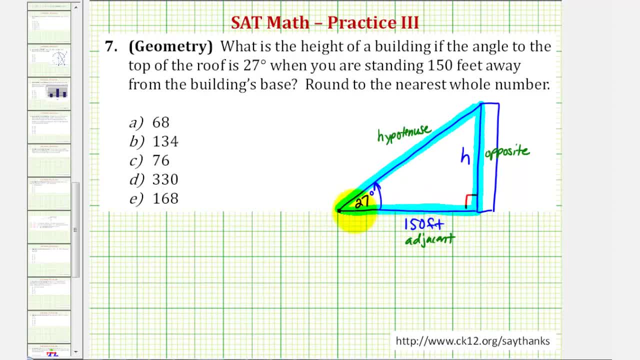 we should recognize that we want to use the tangent function, because tangent theta is equal to the ratio of the opposite side to the adjacent side, Which means we can write a trig equation where tangent twenty-seven degrees must be equal to the ratio of the opposite side to the adjacent side. 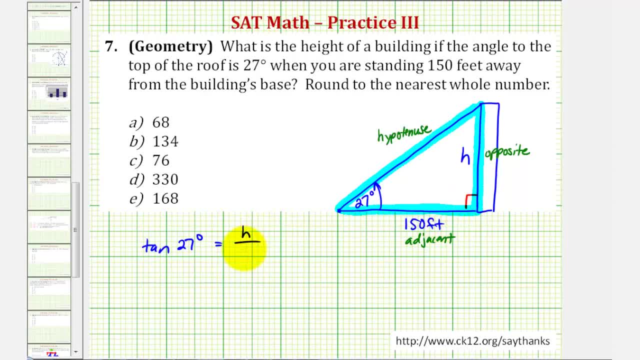 or in this case, h divided by one hundred fifty feet. And now we can solve this equation for h to determine the height of the building. So to solve for h, we want to clear this fraction by multiplying both sides by one hundred fifty. 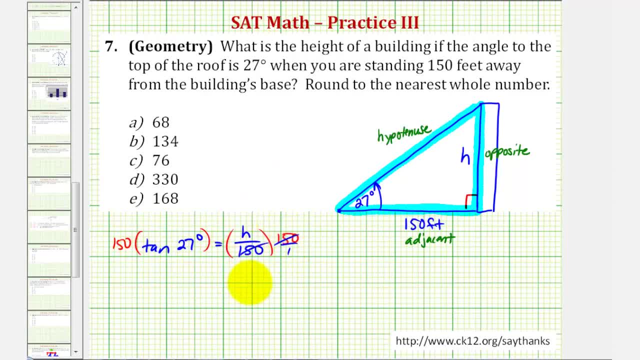 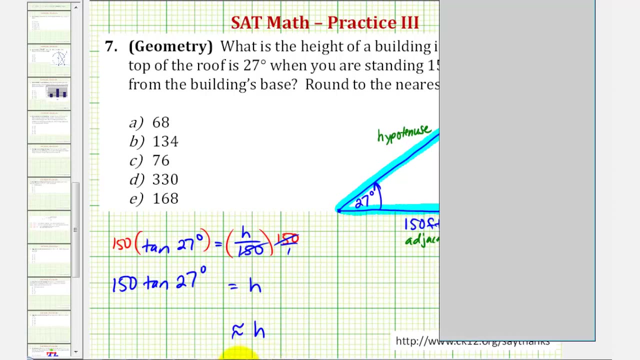 Notice on the right side. this simplifies nicely to h. So h is equal to one hundred fifty times tangent twenty-seven degrees. So now we'll go to the calculator to approximate h to the nearest foot. It's important that we make sure that we are in degree mode, So let's press the mode key. 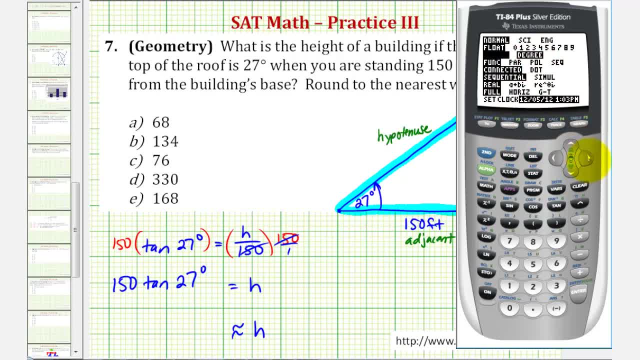 Notice how, on the third row, degree is highlighted. If it wasn't, we would highlight it and press enter. Now we'll go back to the home screen by pressing second mode for quit And we'll type in one hundred fifty tangent twenty-seven degrees. 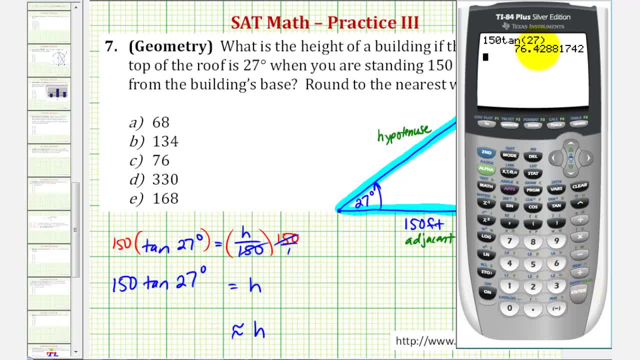 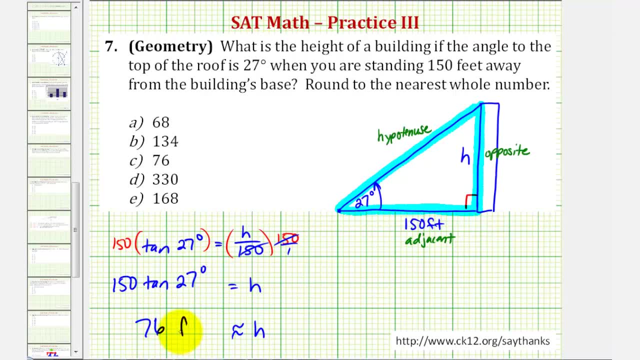 Going to the nearest whole number, the four in the tenths place tells us to round down, And therefore h is approximately seventy-six feet. Therefore, our answer is c seventy-six. I hope you found this helpful.